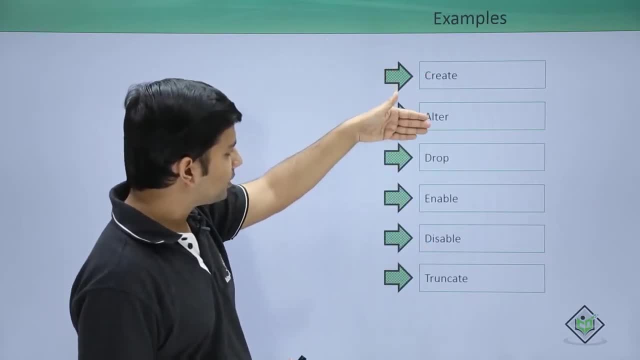 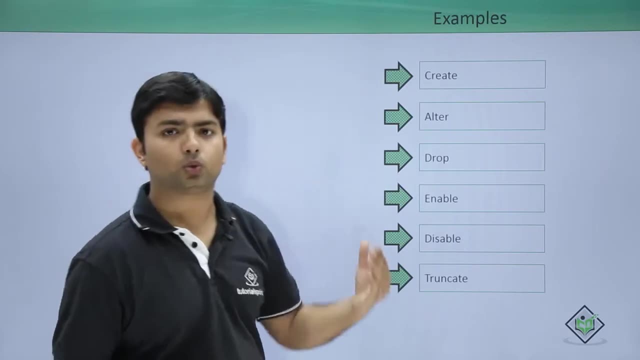 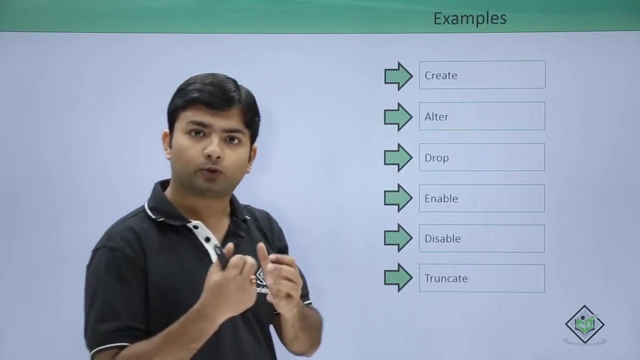 Like here. you can see create, alter, drop, enable, disable and truncate. So whenever you will create a new database object that will be a create keyword will use a create keyword so that create statement will actually create a new database object. initially we will just begin with the table, but in our coming 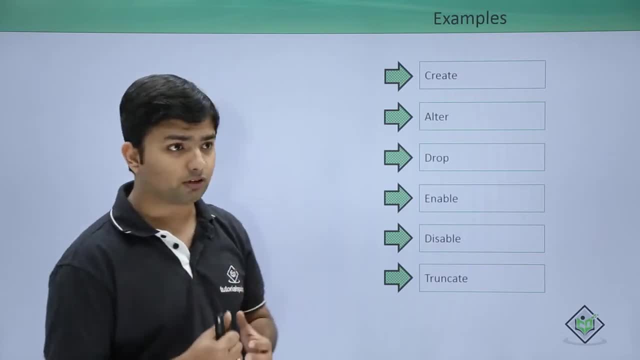 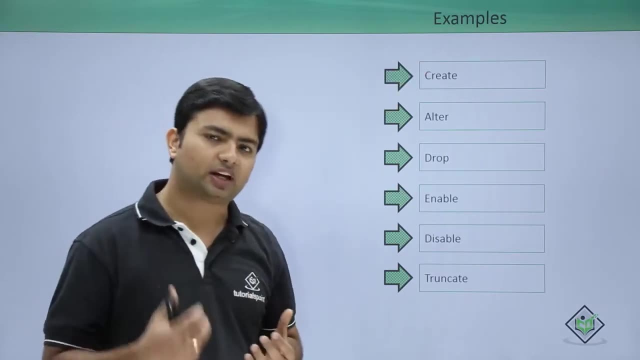 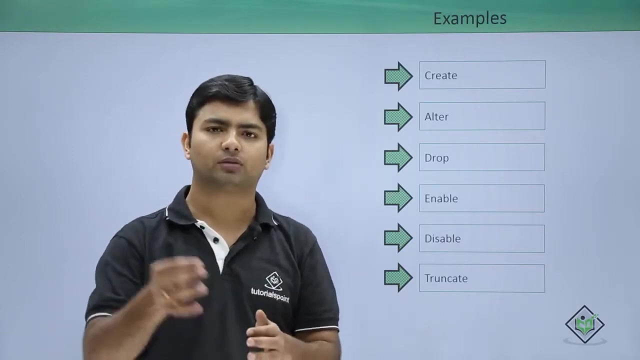 videos. we will cover some more database object and we will find how can we create the different type of database objects using this command. once you have created an object, you want to change the structure. for example, you have created one table. you want to add one more field later. so you can do that by using 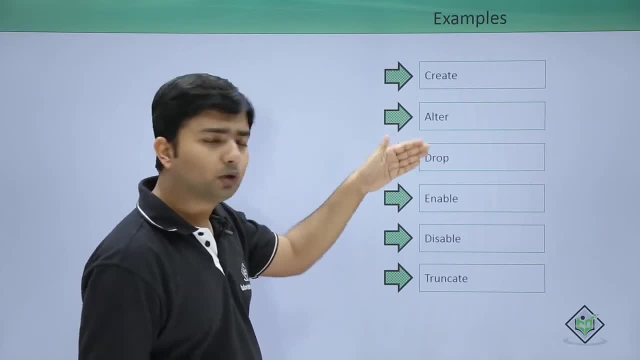 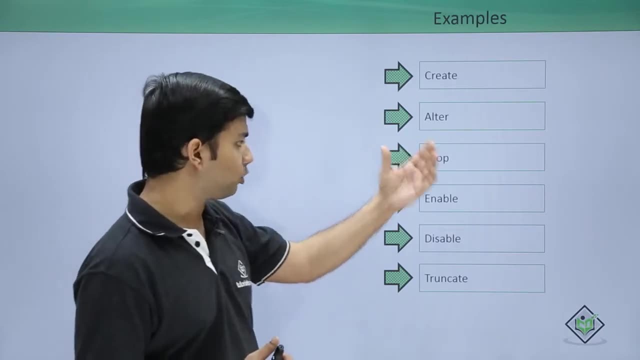 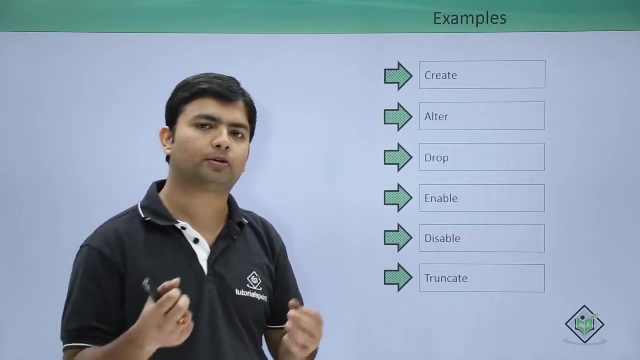 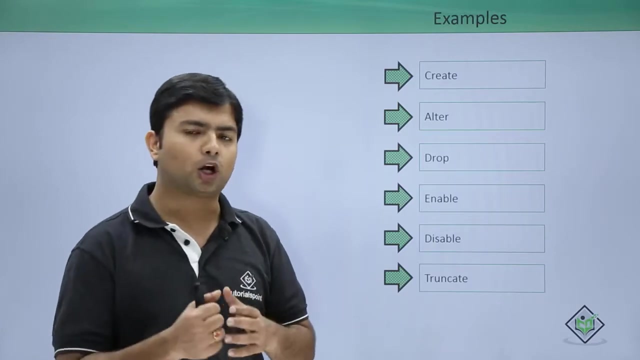 the alter keyword drop will be used to delete the definition and the structure of the database object. if I say drop table TBL employees, that means the table, along with the structure and data, will be dropped permanently. as earlier I said in this video, like these commands are auto committed, you will not. 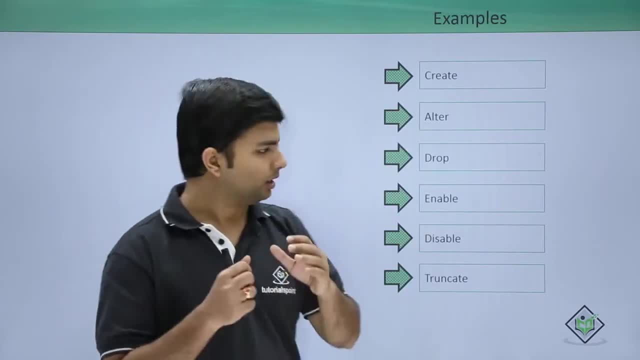 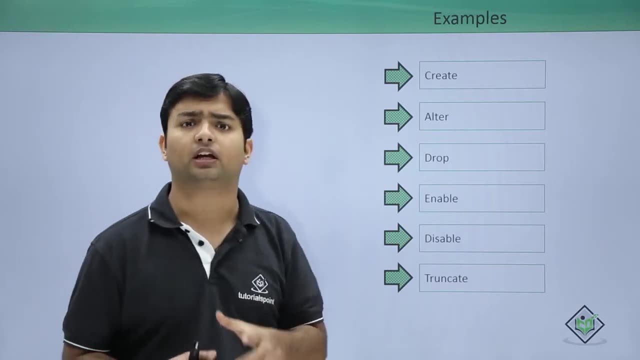 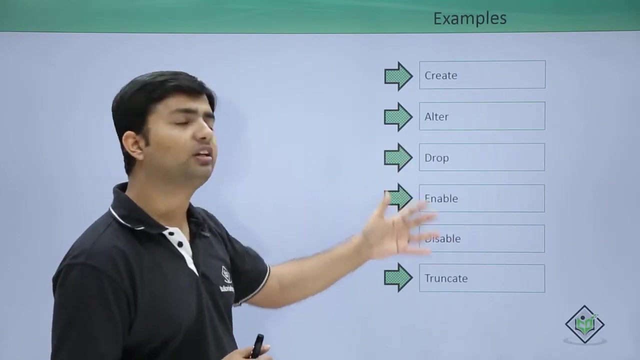 be able to do the undo for such things. now, enable and disable- these couple of commands will be used only for a specific database object called triggers, which we will cover later. but obviously when you will enable or disable a particular trigger, it will be a DDL statement you may think, like when we are 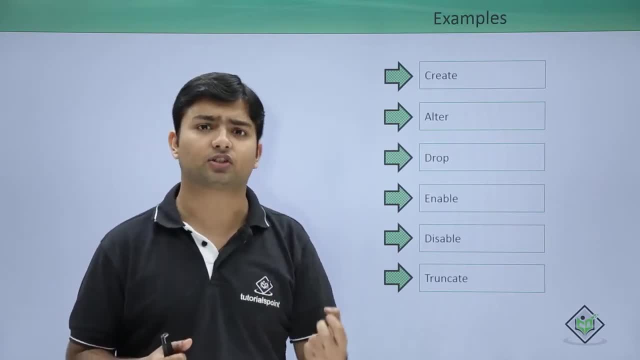 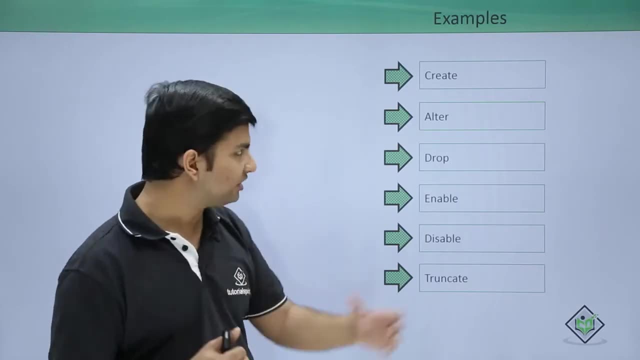 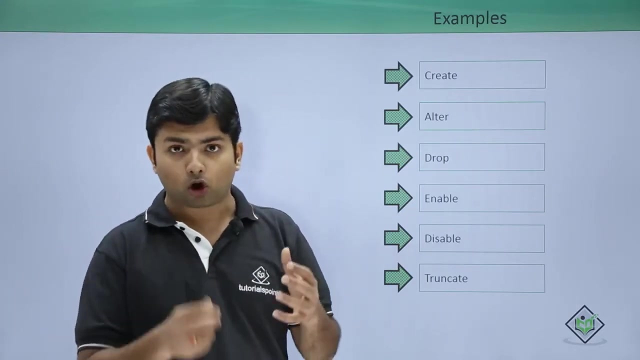 enabling or disabling something. it is not changing the structure because ultimately that particular object, object, like trigger, is still in the database, so why it is inside the DDL? so, as initially I said, any SQL command which will change the structure or the metadata, so here the metadata will be. 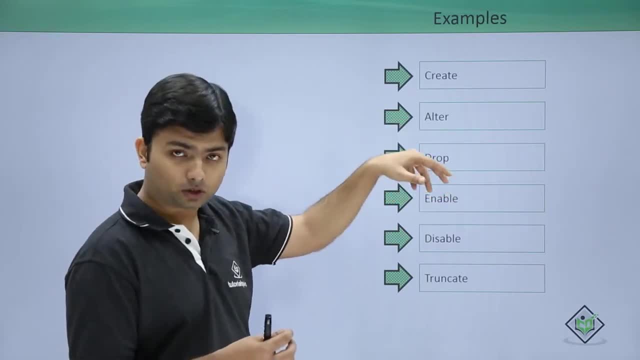 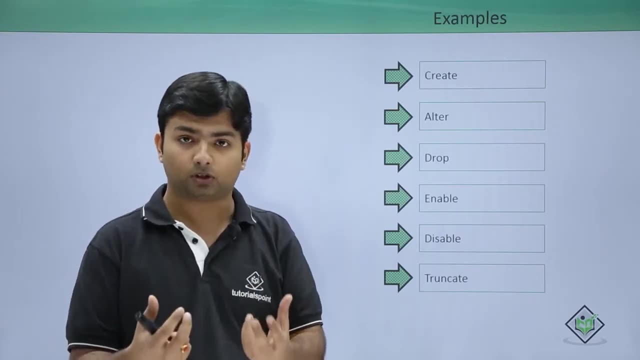 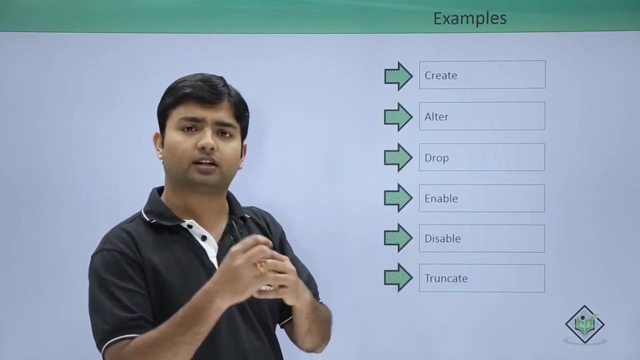 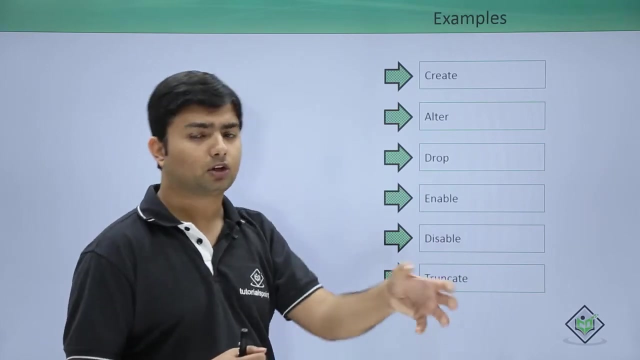 affected. for example, if you will enable or disable a trigger, so in database that particular trigger will not be in action and your table or which, wherever you are applying that trigger, must know that thing. so obviously it will affect the metadata so that the other database objects dependent on that should know that, whether this particular trigger is enabled or disabled, and